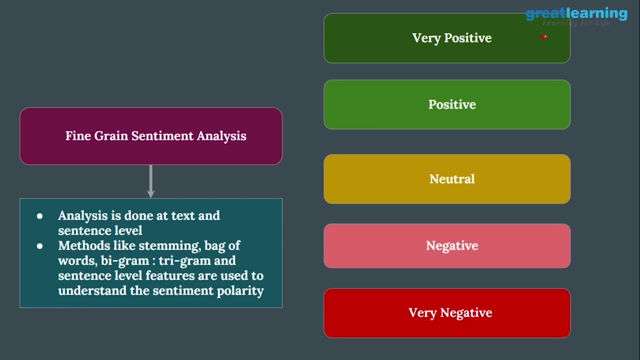 analysis is basically done at text and sentence level. methods like steaming bag of words, bigram, tigram and sentence level features are used to understand the sentiment polarity. maybe your feedback can be very positive, normal, positive, or can be neutral, negative or very negative. so these are the domain or these are the category we have when we are going to check the sentiment for a 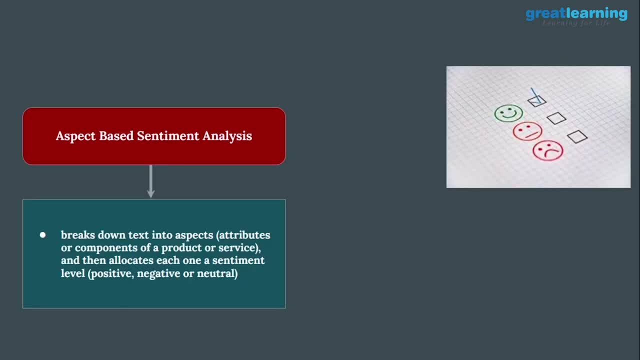 particular review. now let's have a look at what is aspect-based sentiment analysis. so this breakdown stakes into aspect, that is, attributes or components of a product or service, and then allocates each one a sentiment level. may be positive, negative or neutral. so this is how our aspect-based sentiment 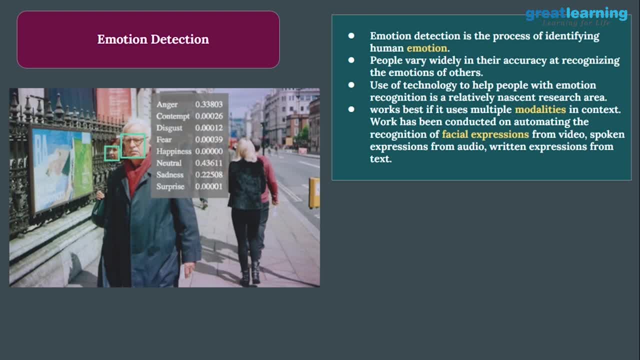 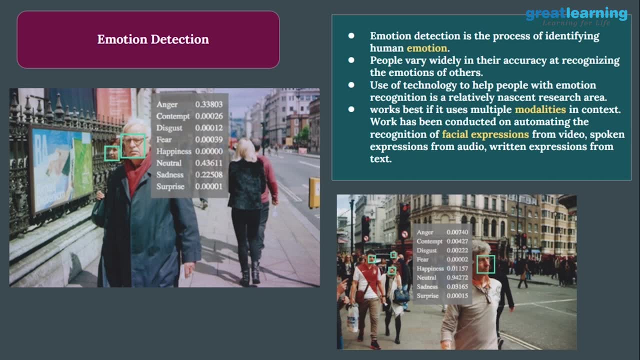 analysis works. now let's have a look at what is emotion detection? from the name itself, you can understand we are going to speech our emotion by looking at the person. so how can you do that? so emotion detection is the process of identifying human emotion. people vary widely in their accuracy at 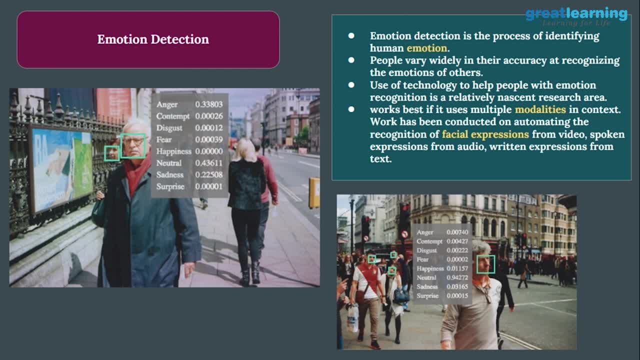 recognizing the emotions of others. use of technology to help people with emotion. recognition is a relatively nascent research area. works best if it uses multiple modalities. in context, work has a conducted on automating the recognition of facial expression from video, spoken expression from audio and reading expression from that. 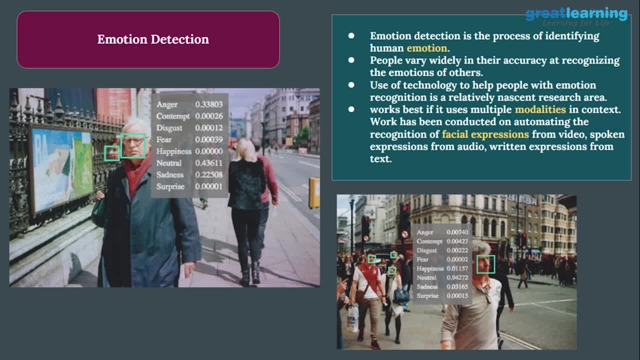 takes. so this is the way you can protect the emotion for a particular person. so you can see in the Disney power program videos, angleacağım apropos high probability of never sadness and all right from this you can see Main生 a pose is neutral because a fancy this and that number. we are. 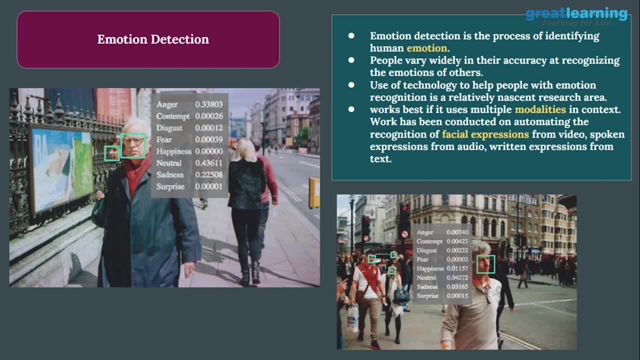 getting over you at the other program with this, looking at the probability of these is nobody. robility is forward robility, hi is for neutral. so you can see this particular person emotion is neutral. so in the second case also, you can see the neutral probability is 0.9. so in this case we can quite sure that. 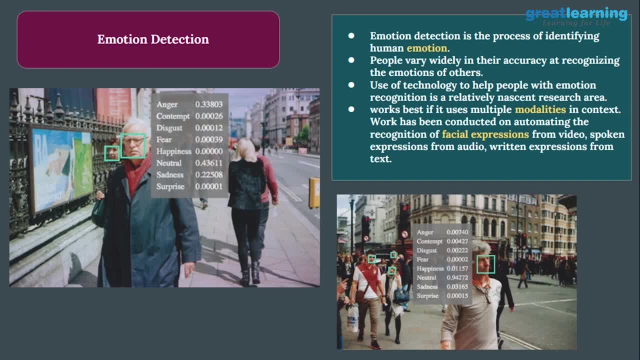 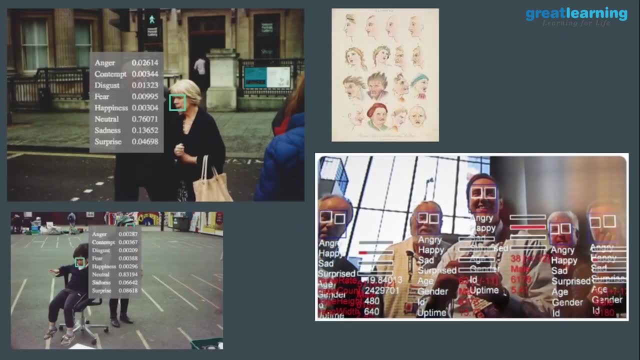 this person, emotion is neutral. so this is how we actually go for detecting the emotion for that particular person. we'll have a look at other ways of doing that. maybe. here you are getting another applications of angry, happy, sad, surprise. so it's up to you. what are the emotions you want to add to your application, right? so these are the main, or 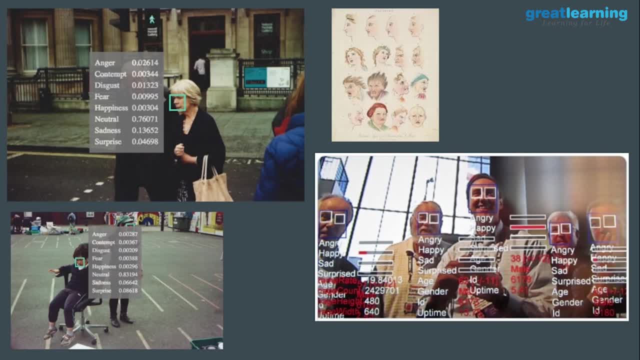 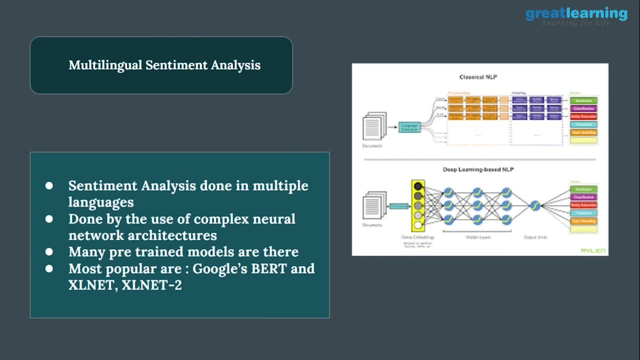 you can say these are the one of the best use of sentiment analysis. now we will have a look at multilingual sentiment analysis. but what is multilingual sentiment analysis? the sentiment analysis done in multiple languages, done by the use of complex neural networks architecture like RNN, LSTM. many pretend models are there, so pretend models are basically. 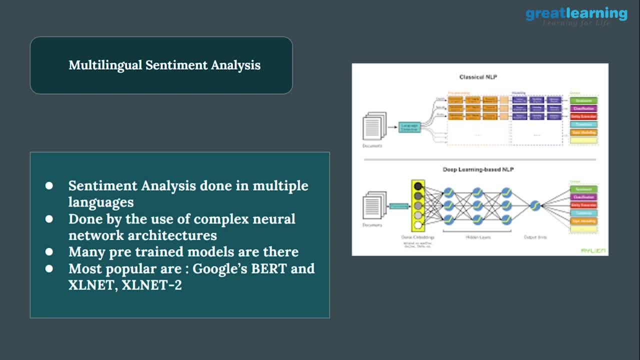 the models who are used to detect the emotions of the person, and what are the emotions that you want to add to your application? right? so these are the main. or you can say: these are the models who are trained with a huge number of data sets. so in that case, when you are 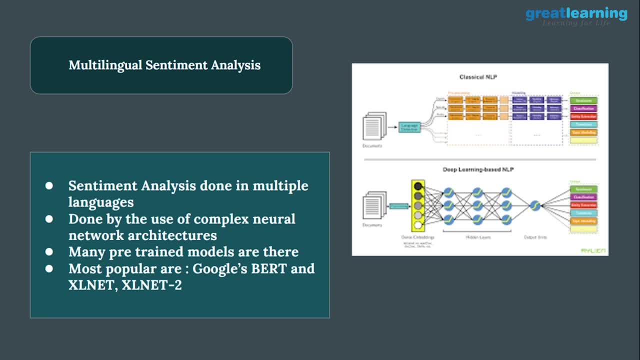 you are going to use a pretend model, you don't need to write a model from a scratch. what you need to do, you can just change the output layer according to your users. so most popular trained models: we have google's part and excel net, excel net 2 as well. so these are the pretend 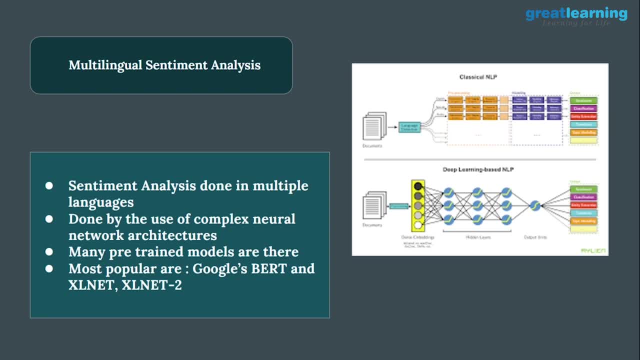 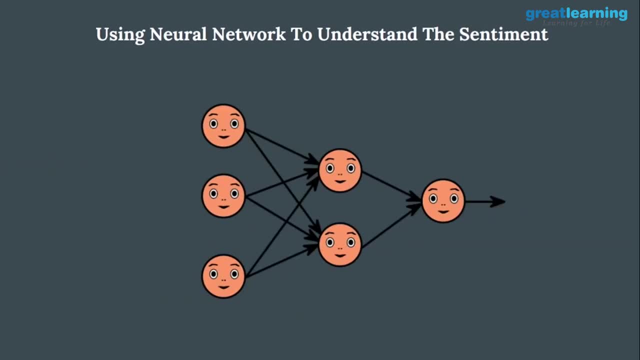 model option you have if you want to make a pretend sentiment analysis model, and that is what we are going to do, that as well. now we are going to talk about neural network, so we can do this sentiment analysis using machine learning as well. but if you want to, 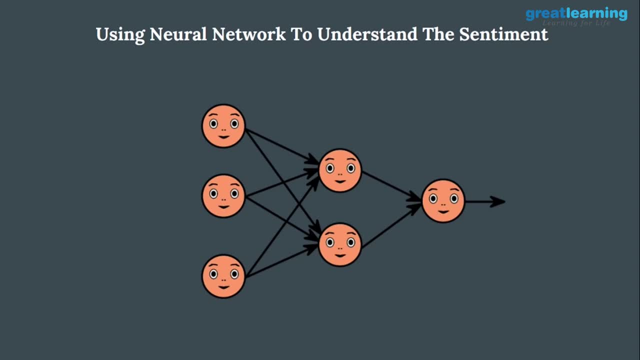 make the sentiment analysis in an advanced way, that time you need to go for neural network. but what is that neural network stands for? basically, neural network is like a replica of human being, but the scientists try to make a replica of human being which can detect and work like a human brain, right? so there are lots of algorithms that can be used to. 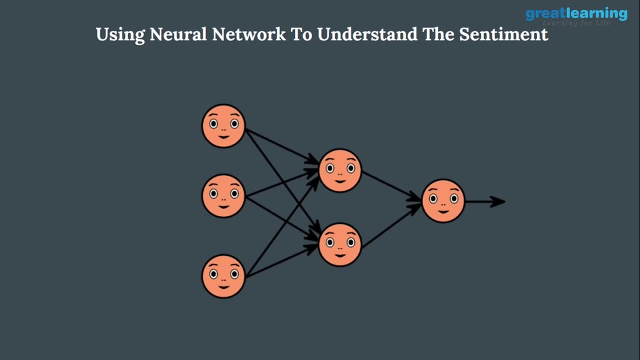 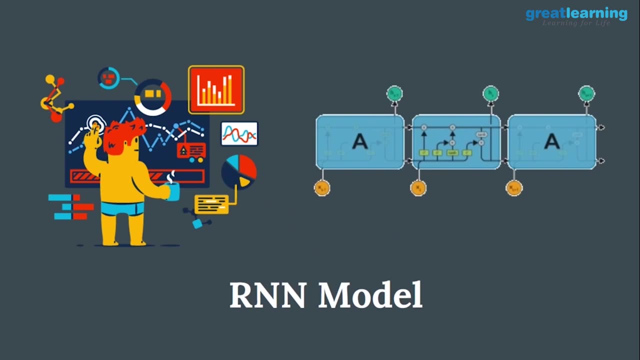 detect human beings and lots of parts we have in neural network. who can do the sentiment analysis like a human? now we will have a look at rnn model. so basically, rnn stands for recurrent neural network. so we use recurrent neural network model to do the sentiment analysis and this model is quite familiar to work with the sequential model as well. but why i am? 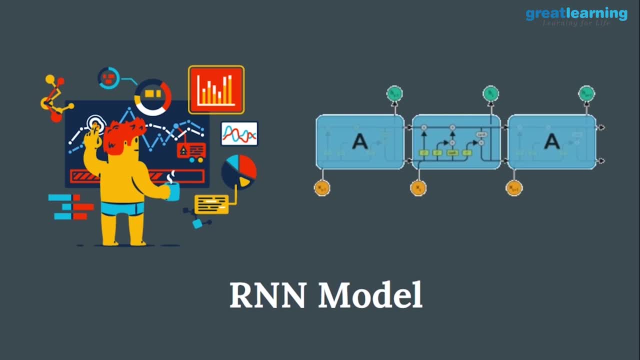 talking about sequential model because the sequential model does maintain the insertion order. so whenever you are going to make a sentiment analysis, you need to make a sentiment analysis for a particular sentence. you need to maintain the sequence as well. so this is how rnn model is recommended for sentiment analysis case. now we have lots of other algorithms.